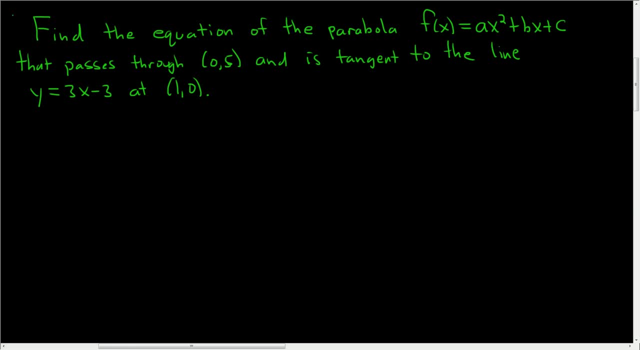 Find the equation of the parabola that passes through the point 0 comma 5 and is tangent to the line y equals 3x minus 3 at 1 comma 0. solution: Let's go ahead and write down everything that we're given. So we're told it passes through 0 comma 5.. That means that f of 0 is equal to 5.. 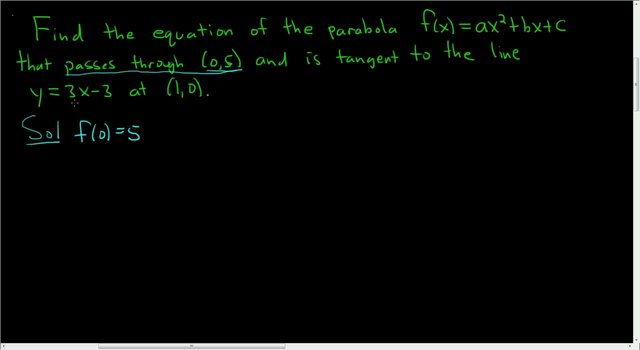 Okay, we're also told it's tangent to this line at 1 comma 0. That means that f of 1 is equal to 0 because it passes through 1 comma 0. And it also means that the derivative of f at 1 is equal to 3 because the derivative of f at 1 is the slope of the tangent line when x is equal to 1. and that slope 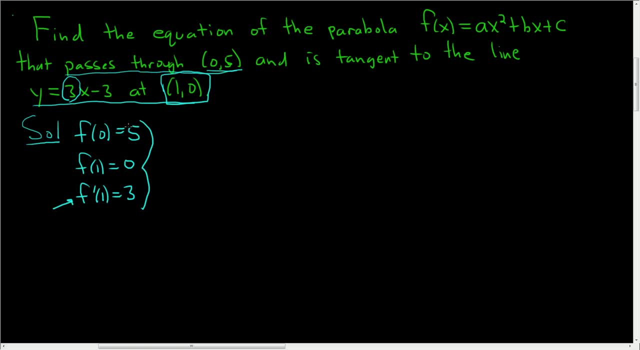 is 3.. Now that we've written down all of the information, let's just go ahead and use it to find a, b and c. So we'll start with the first condition. So f of 0 equal to 5.. So we get a times 0 squared plus b, times 0 plus c, and that's equal to 5.. 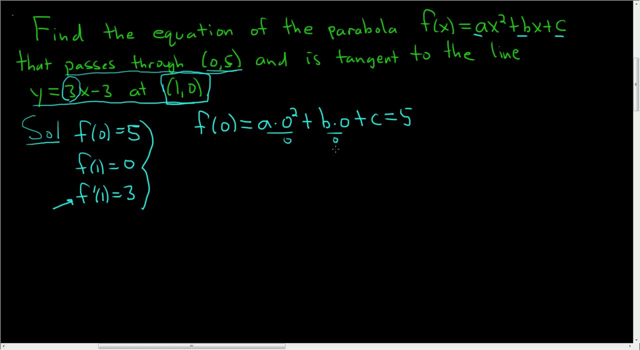 So this is the equation of the parabola that passes through the point 0, comma 5.. This is 0,, this is 0, so we end up with c equal to 5.. So we have one of our constants. So f of x can be rewritten now as ax squared plus bx plus 5.. 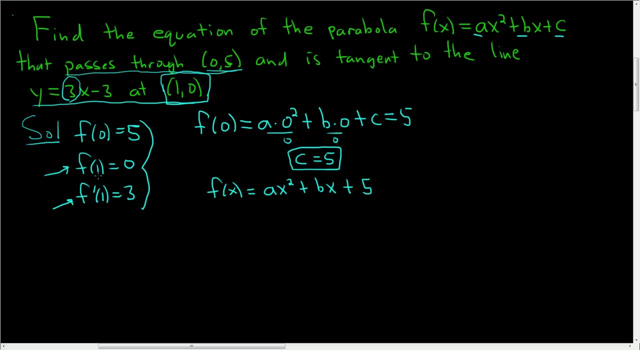 To use the next two conditions. well, to use the next one, we can just plug in 1, and then to use the third one, we have to take the derivative. go ahead and take the derivative. So f prime of x is 2ax plus b. right, The derivative of bx is b. 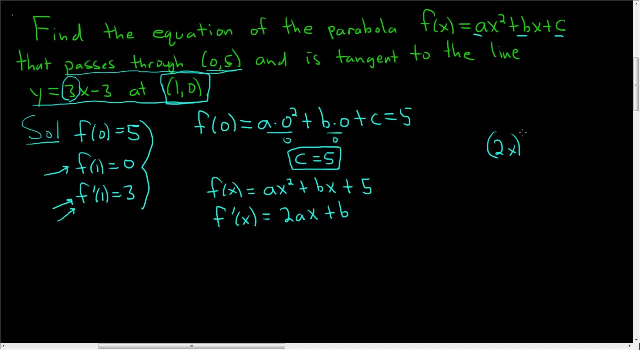 right. Think about this: The derivative of 2x is 2.. The derivative of 3x is 3.. So the derivative of bx is just b. b is a constant And the derivative of 5 is 0. So we didn't bother writing it, Let's.